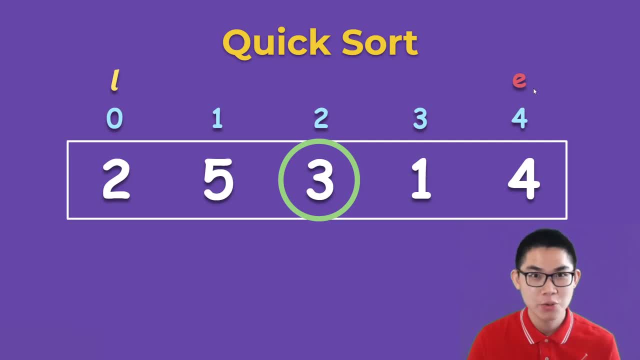 So we replace s with l and e with r, And the goal of this game is to do something called partition, and I like to think of it as a game with two players. The last step of the game is to get all the numbers less than the pivot on the left bubble. 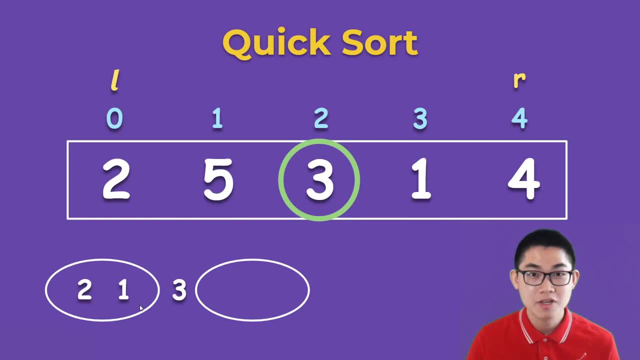 So, for example, here we have 2 and 1, and all the numbers larger than the pivot to the right bubble, so 5 and 4.. Here the order does not matter, as long as you get the numbers in their correct places. 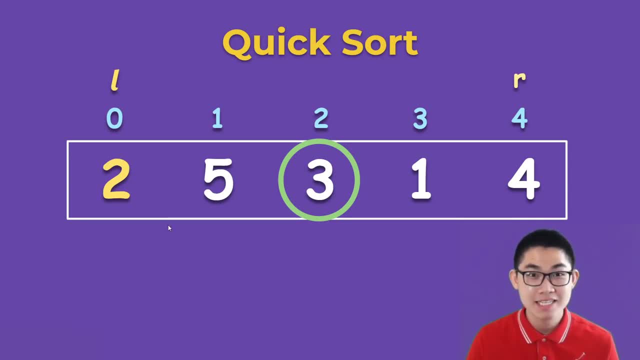 So the player l will find us a number that is larger than the pivot or equal to the pivot. So let's see No, Yes, Because 5 is larger than the pivot. now r will find us a number that is either smaller than the pivot or equal to the pivot. 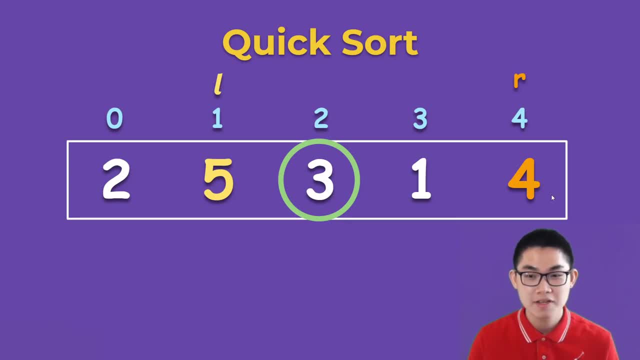 so, nope, four is not smaller or equal to the pivot. so let's take a look at one. and yes, it is. one is smaller than three. and what to do next? well, we simply swap five and one. so now you see that one is in the left bubble and five is in the right bubble, and then we move l to the right. 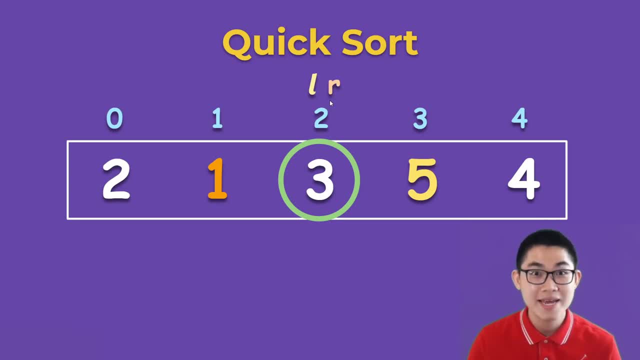 and r to the left and repeat this process. remember, l will try to find us a number that is larger than the pivot or equal to the pivot, and l already found three. right, it's equal to the pivot. now r will find us a number that is smaller than the pivot or equal to the pivot, so r also finds. 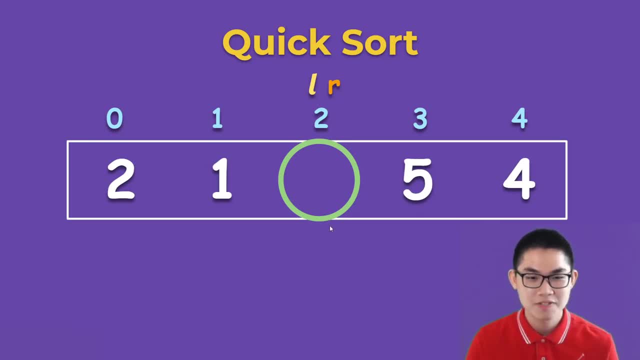 three and we swap three with itself. so just swap in place and then we move l you the right and r to the left. at this point l and r have crossed each other and this indicates that the partition game is finished. so notice that all the numbers smaller than 3 are to the left side. 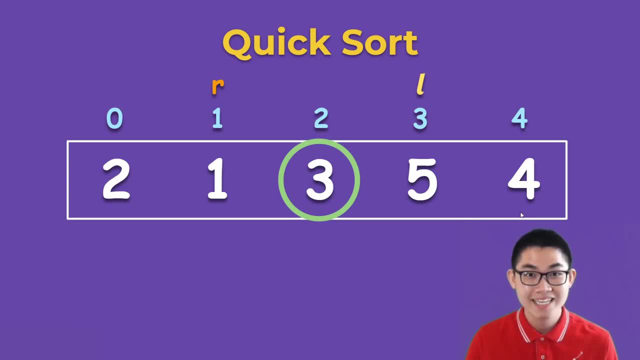 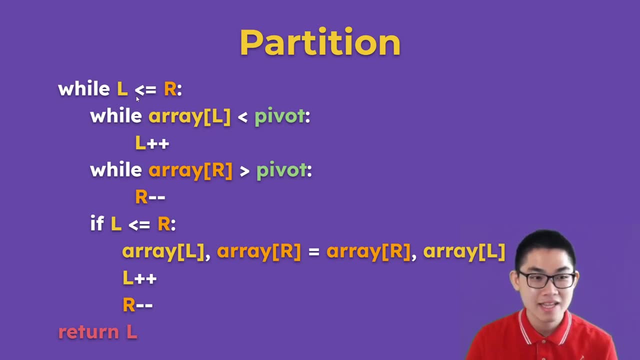 and all the numbers greater than 3 are to the right side. before we move on to the next step, let's first summarize the partition game. so, while l is less than or equal to r, basically this just means repeat these following steps until l and r cross each other, and that's when the game finishes. 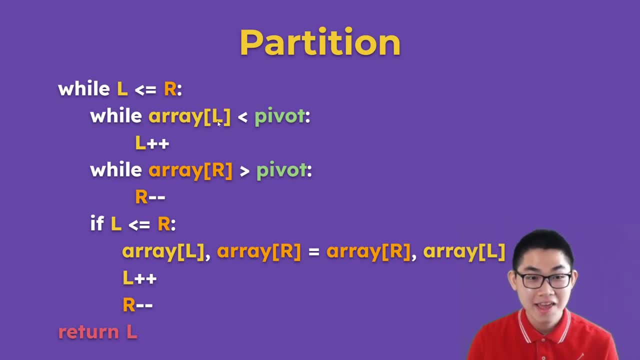 while the number in the array at l is smaller than the pivot, we move l to the right. so after this while loop, l will find us a number that is either larger than the pivot or equal to the pivot. now the next while loop. so, while the number in the array at r 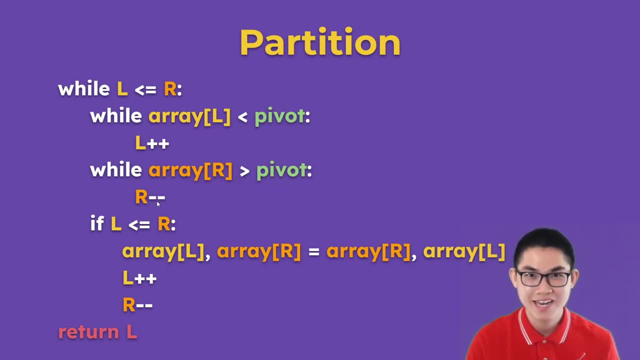 is greater than the pivot, we move r to the left. so what is the result after this? while loop? well, r will find us a number that is either smaller than the pivot or equal to the pivot, and we're almost done. so we check. if l and r have not crossed each other yet. then we swap the numbers. 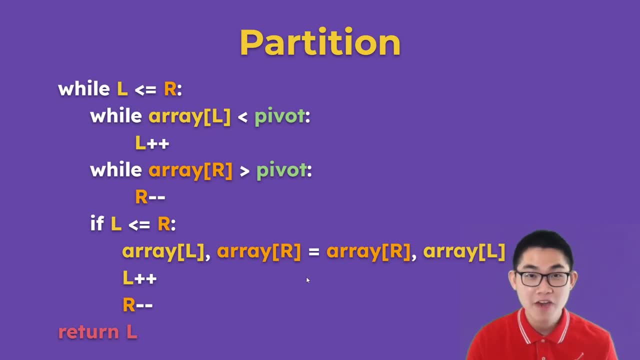 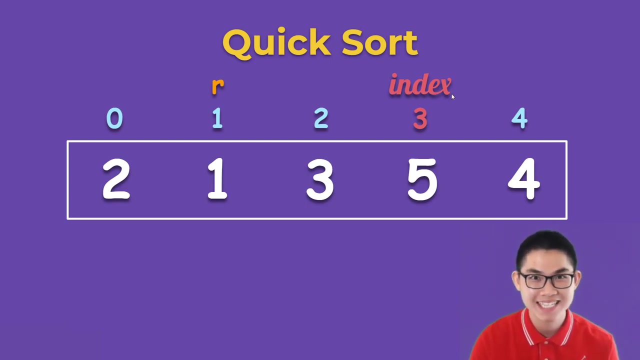 in the array at index l and r, we move l to the right and r to the left, and the last step is to return l. and i'll show you what's going to happen. so, basically, l was here before. we just replace l with a different variable called index. and why do we do this? well, remember, we want to. 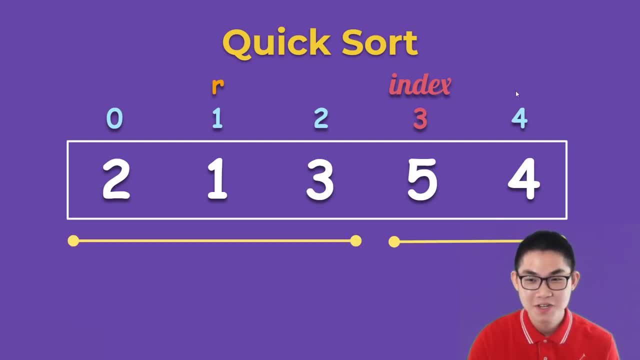 partition. the array right, so from the index to the end of the array- will be in its own box, like this, and the other side will also be in its own box. now, quick sort is recursive in nature, so basically we repeat quicksort on top and bottom, and then we'll have this as the new variable, and then we'll have 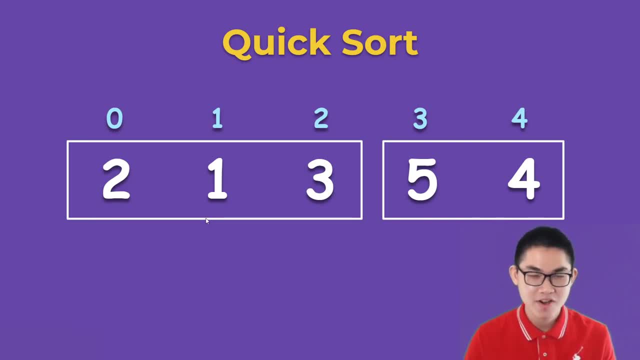 the left side first and then on the right side, So always on the left side. we put S, which is the start, and then E at the end. We calculate the mid. so S is 0, E is 2, so we get 2 divided by 2, which gives us 1, and then at mid we have the. 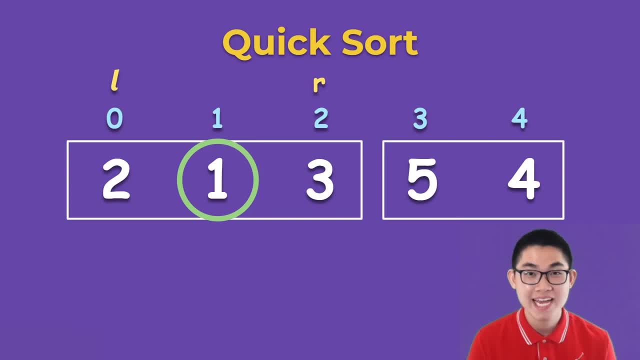 pivot. Once we have the pivot, we're going to play the partition game. So L will find us a number that is either larger than the pivot or equal to the pivot. Yep, we found it. 2 is larger than 1, which is the pivot. Now R will find us a. 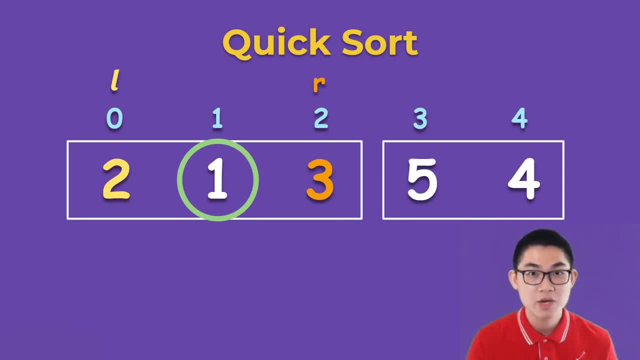 number that is either smaller than the pivot or equal to the pivot. So, nope, at 3, it's not At 1. yep, we found it because 1 is equal to the pivot. and then we swap the numbers in the array at L and R. So just like that. Finally, we move L to 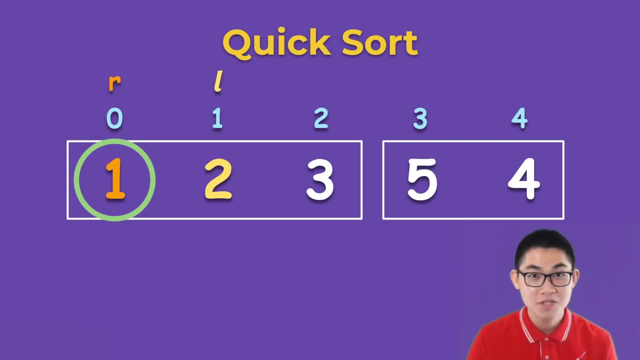 the right and R to the left. Notice that L and R have crossed each other, which means that the partition game is now finished. We replace L with another variable called index and basically, from the index to the end of this box will be in its own separate box. 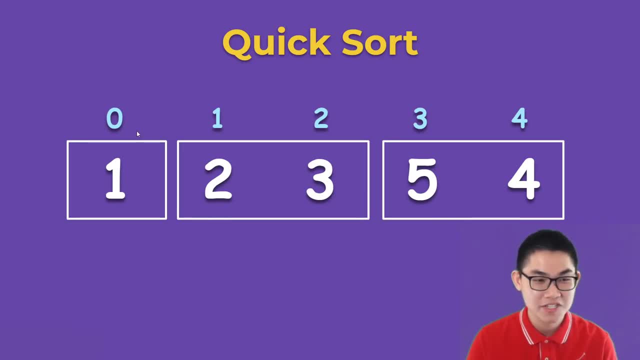 just like that. We look at the leftmost box and place the start and the end onto this box. Now, when the start and the end are on the same number, this indicates that this number is the same number as the start and the end of the box. So we 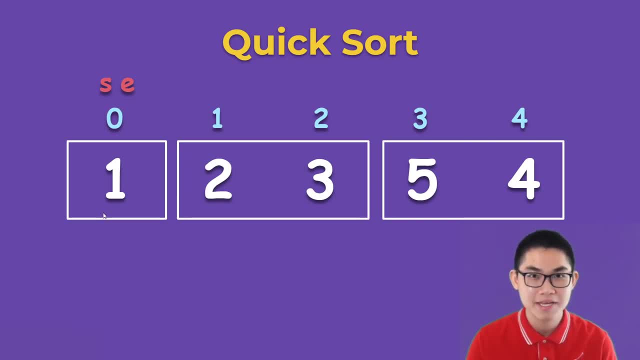 place the start and the end on the next box. We calculate the mid. So S is 1.. E is 2.. So 1 plus 2 gives you 3.. 3 divided by 2 gives you 1.5.. And these signs means you round. 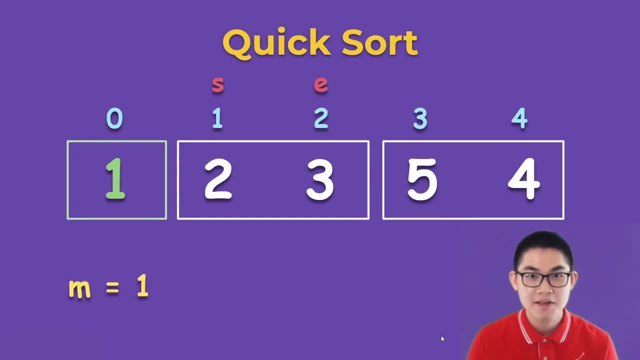 down. So 1.5 rounded down gives you 1.. Mid is at index 1. And 2 will be at index 2.. So 2 will be our pivot. Now we play the partition game, So L will find us a number. 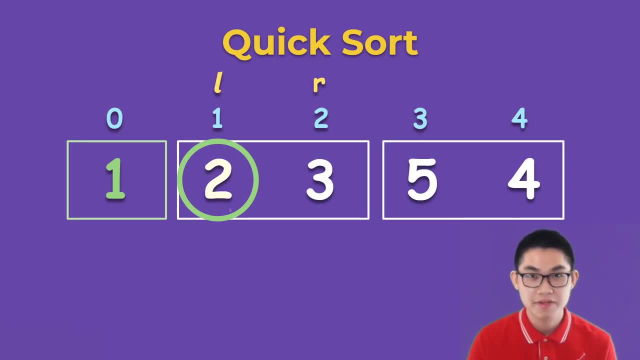 that is either larger than the pivot or equal to the pivot. We found 2, and 2 is equal to the pivot. R will find us a number that is smaller or equal to the pivot. So 3 is not, 2 is yes, because 2 is equal to the pivot. Then we swap the. 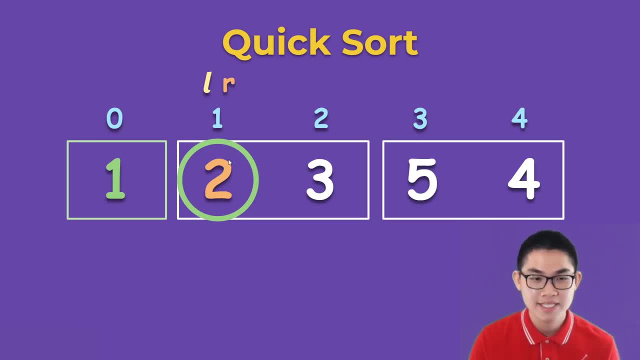 number in the array at index L and R. So basically just swap 2 with itself And then we move L to the right and R to the left. At this point L and R have crossed each other, which means that the partition game is finished. We replace L with the variable. 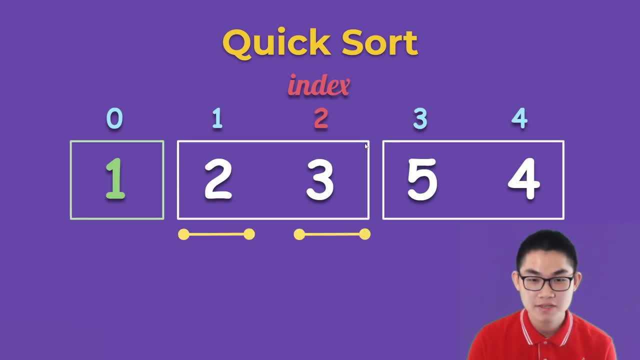 index and from index to the end of this box, like this, will be in its own separate space. We put S and E on this box And since S and E are on the same number, this indicates that 2 is also in its correct place. 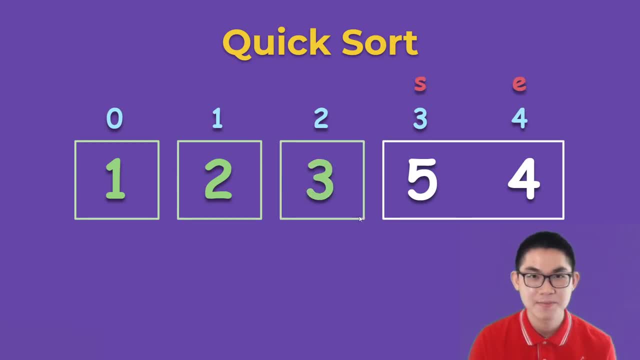 Now we look at this box And it's also in its correct place. Now our last box. So we calculate the mid. So we have 3 plus 4, which is 7, divided by 2, which gives us 3.5. Round.